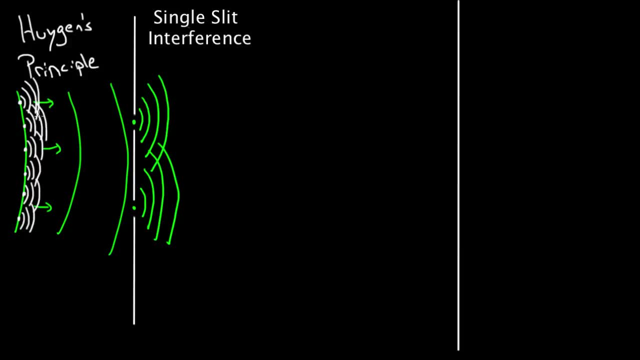 of another wave And you're thinking this is horribly complicated. What, What kind of mess is this going to give you? Well, if you add this up, these are going to interfere with each other- Constructive, destructive- In a way that just gives you this same wave. 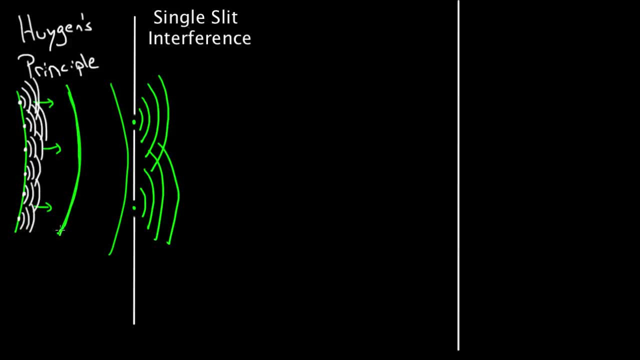 front right back. This is crazy But true. If you let every point on this wave be another wave source, it will just add up to another wave front. here You'll just get the same thing back. And this is the key to understanding why diffraction happens Is because the wave spread. The wave was already. 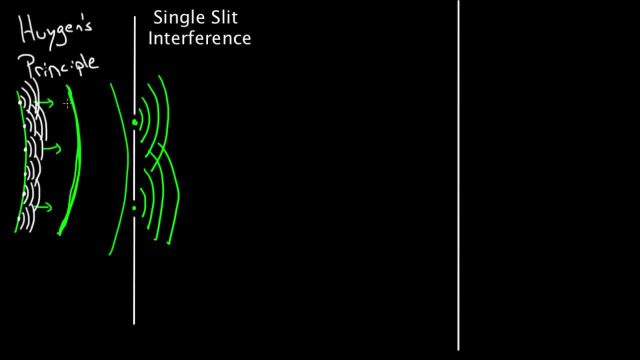 diffracting, so to speak. It was already doing diffraction. Every point on here was doing diffraction, It's just. it always added up with the other waves around it at every other point. but when there's a barrier, when there's something in the way these here can't. 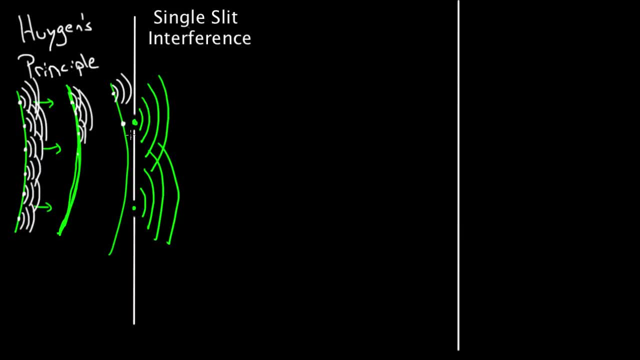 rejoin up with their buddies. you just get this one here spreading out and then this one down here spreads out. all the rest of these get blocked. now that these are blocked, they're not going to get to interfere constructively and destructively with these points here. and so what do you see when it hits the hole? 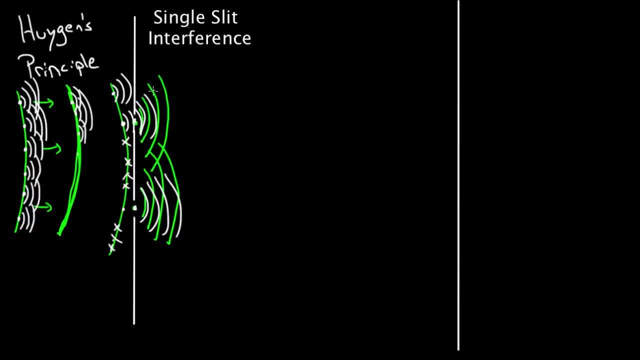 you just see this thing spreading out, so it was always diffracting, so to speak. we just didn't notice it, because it always added up when you've got a hole or a barrier, that's when we actually notice it. and this is the key to single slit. 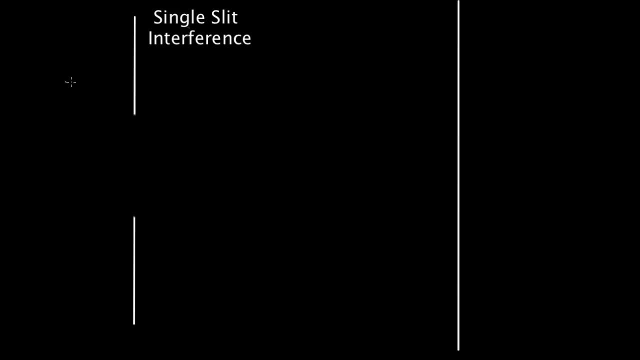 interference, because if I get rid of all that, if we imagine our wave coming in here like this, well, this wave is going to hit here. every point is the source of another wave, so this point is going to start spreading out. this point is going to start spreading out. when we have a single slit, we really have infinitely. 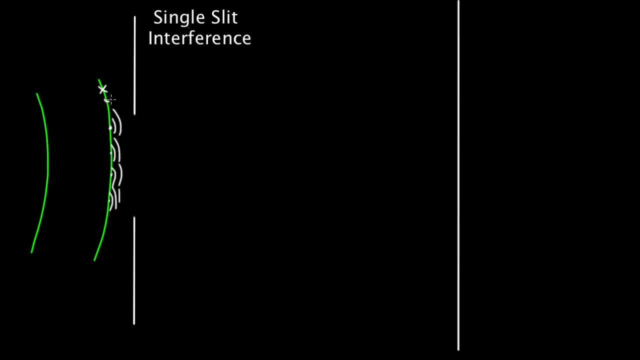 many sources of waves here and since some of them are blocked, we could see an interference pattern over here on the wall, because these can interact and interfere with each other. what interference pattern are we gonna see? well, on the wall over here we see a big old bright spot right in the middle, and if I were guessing I would have thought: 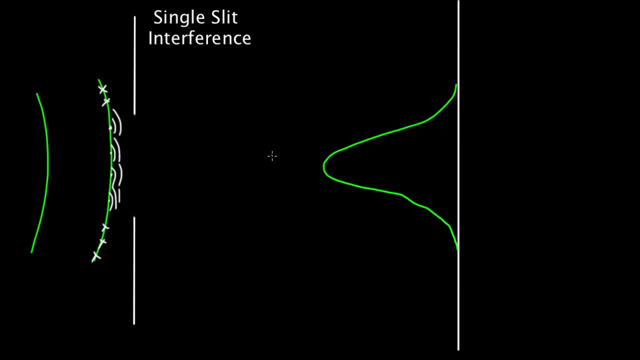 that was it big old bright spot. because you shine a light through a small hole, single hole, you'll get a big bright spot there. the weird thing is this jumps back up, goes to a minimum, a zero point, and then it jumps back up and then it comes. 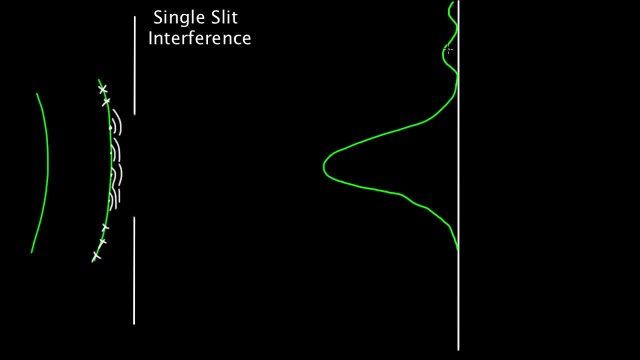 back up again and you get this: these are gonna be not very pronounced, these aren't very pronounced. you get a big bright spot in the middle. these are relatively weak compared to other interference patterns that we've looked at and down here jumps up a little bit again over and over here. so this is the. 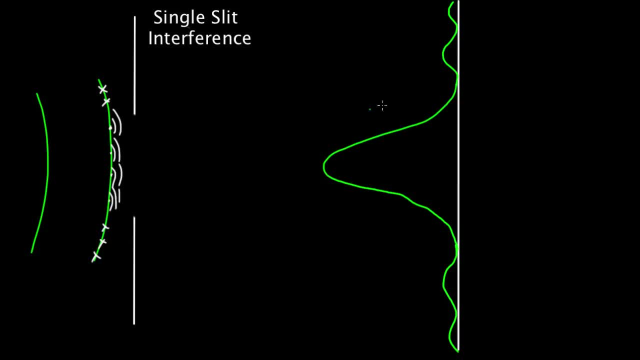 pattern. you see, how can we get this? how do we analyze it? that's what we're gonna try to figure out. to figure that out, okay. well, this is a. I said there's infinitely many sources here with when this wave gets to here. that would take a. 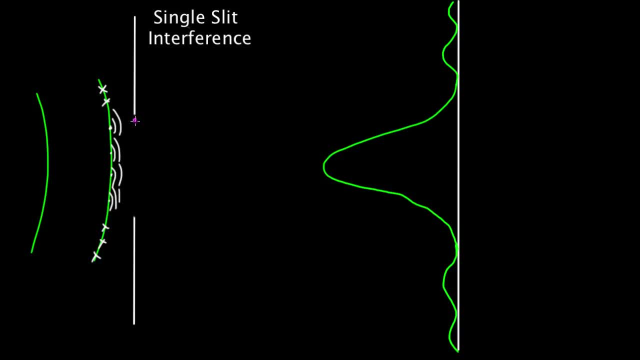 long time to draw. I'm gonna draw eight. so let's say there's one, two, eight sources. let's just imagine there's eight here to make this a little bit easier to think about. and the weird part is that this jumps back up here. so let's look at this minimum. 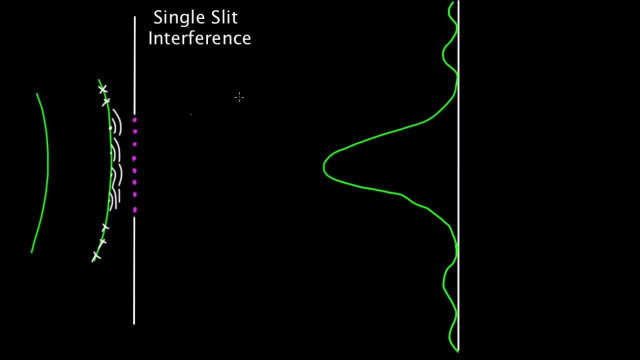 right here. let's look at this point where it goes to zero, this destructive point. so the wave from this topmost point, this wave from the topmost, uppermost point, has to travel a certain distance to get there. I'm gonna also look at the fifth one. 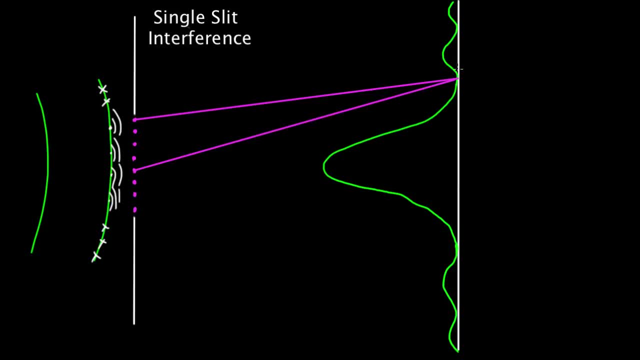 down this one. that's basically halfway. how about these two? if these two interfere destructively? the argument I'm gonna make is: if these two interfere destructively, all the rest of them are gonna have to interfere destructively. why? well, we know how to play this game. let's draw our right angle line here. 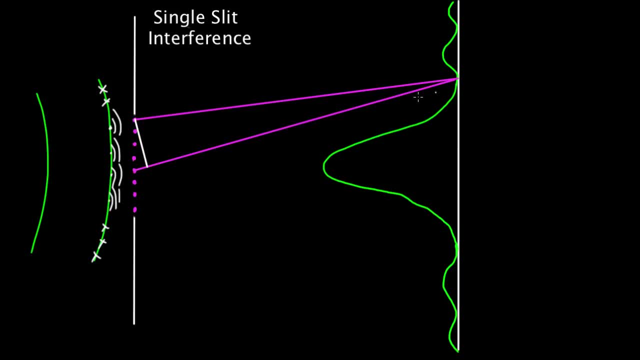 there we go, and so we know that. okay, if these are gonna interfere destructively, this is the extra path length, this extra path length that this second wave, this lower middle wave, has to travel, has to be what? if I want destructive over here, it's got to be a half wavelength, three halves wavelength, five halves wavelength. 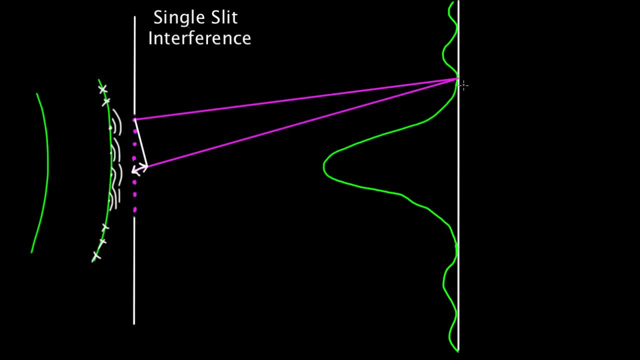 that's how much it's got to be in order to be destructive. so if this is the first point, let's just say that's one half of a wavelength. and what's the relationship between the angle that this is at on the wall compared to the center? 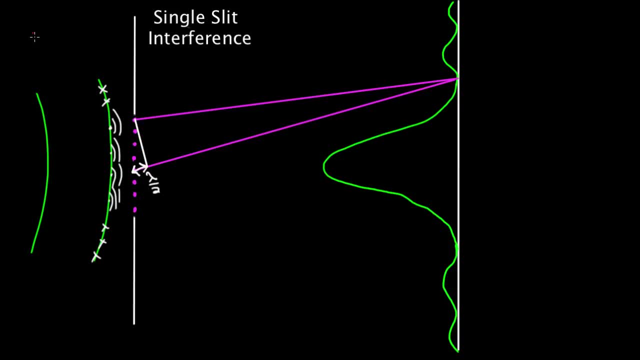 line. well, we already figured that out. remember that relationship was: d sine theta equals the path length difference. between these that we derived the screen had to be very far away compared to the width of the hole, but that that relationship still applies. what would D be in this case? now we have 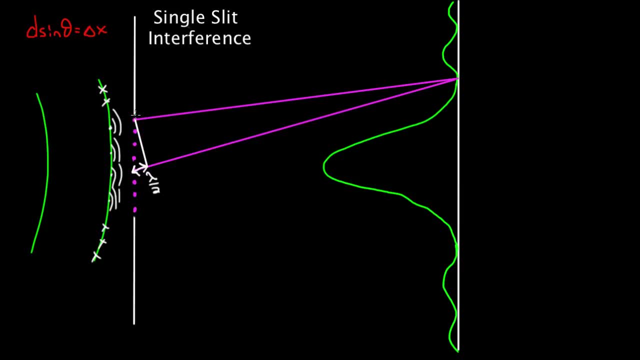 to be pretty careful. you have to be careful because this hole has a certain width. we'll call that width W. so if this hole has a certain width W, how far apart are these? these are not W apart. these are W over 2 apart. and so what's the relationship here? 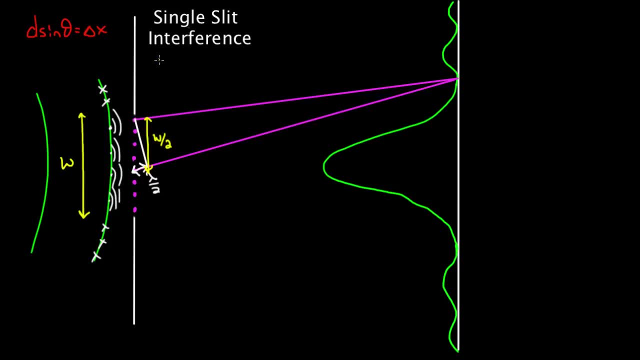 for the path length difference between these two. well, if they're W over 2 apart, I'd have D sine. theta is the path length difference. so D would be W over 2 times sine of the angle that this makes to this point on the wall. and if their path? 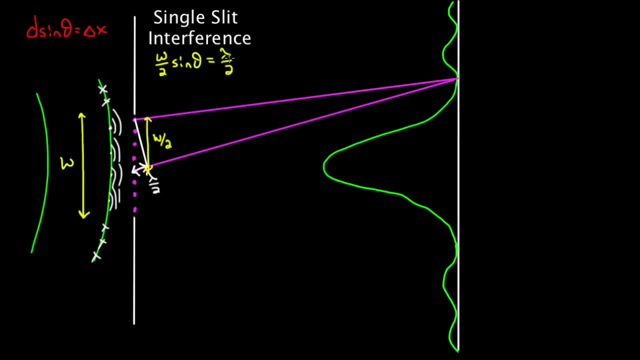 length difference is lambda over 2, then that would be destructive. so equals lambda over 2. and this is a little weird already because, look, I can cancel off the twos and what do I get? I get that W the width of the entire width of the slit times. 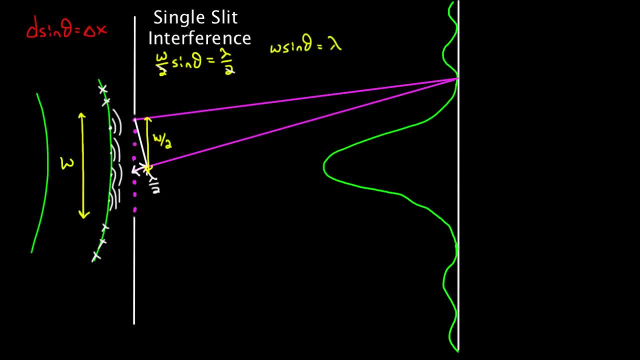 sine of theta equals lambda. this is giving me destructive. remember. before, all the points that were integer wavelengths were giving me constructive. this time it's giving me a destructive point over here and the The reason is we played this game where W is the whole width. These are only W over two apart. 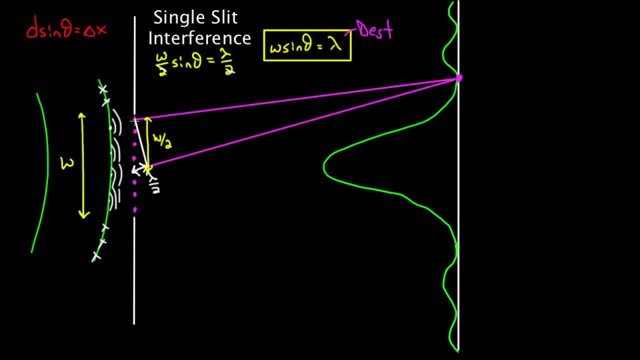 That two cancels with that two. Okay, but I haven't really proved that this whole, that they should all be destructive. yet This is just for these two. We've got infinitely many more in here. How are we ever gonna show that if these two cancel? 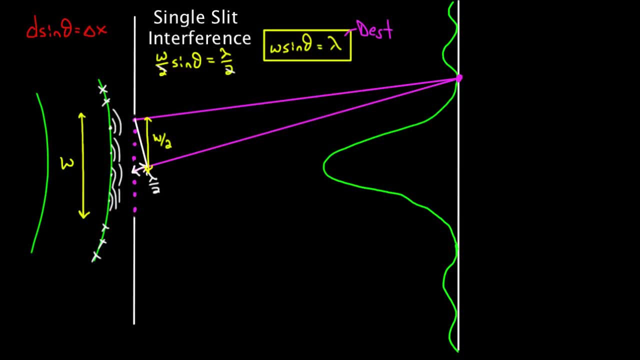 the rest of them cancel. Well, we'll just pair them off. Look at this Now. imagine you come down one. I go to this one. I consider this wave that makes it over to here And then the next wave down from this other one here. 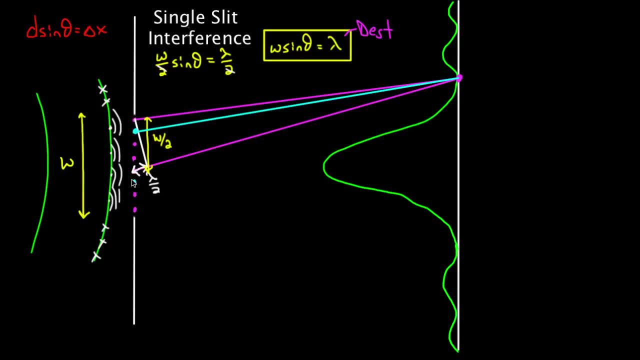 So I move this one down a smidgen, I move this one down a smidgen, and I imagine these two waves traveling a certain distance to get over to this point. What relationship holds between these two? I can do the same thing. 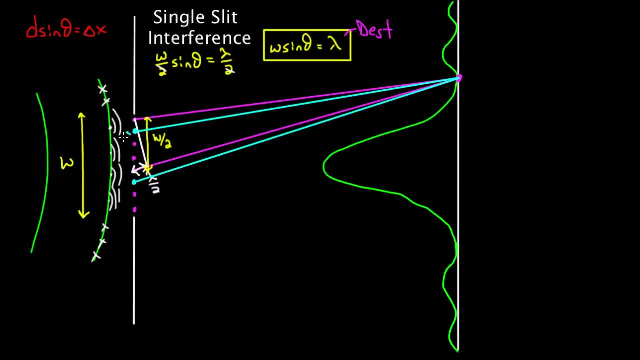 These are also W over two apart. So this here is also W over two. So I'd get the same relationship. I'd get W over two sine of, W over two sine of W over two sine of. is that gonna be the same angle? 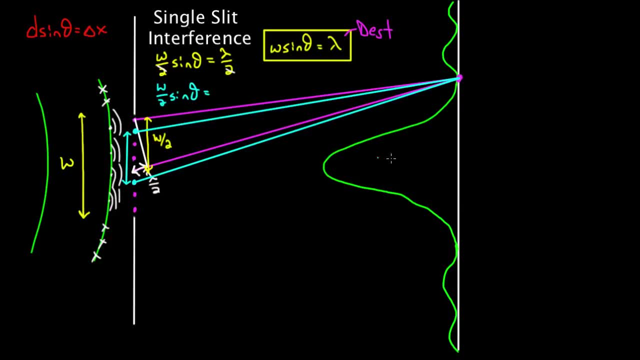 Yeah, it's the same angle, same point on the wall. This is really far away. so these approximations are whole where these lines are supposed to be approximately parallel, because this screen or this wall's very far away compared to the width. 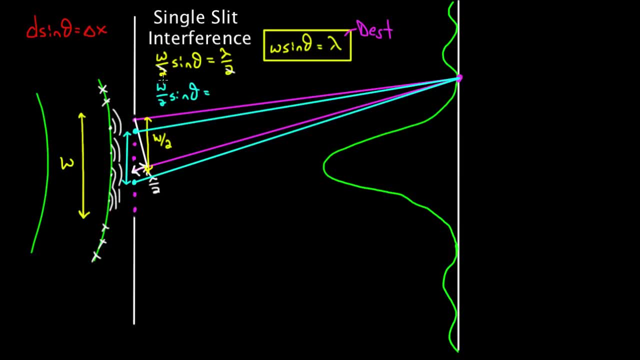 That equals. well, that's gonna be the same thing. I got W over two times sine of the same angle Shoot. that's gotta equal the same thing that it did up here. If the angle's the same, my W over two is the same. 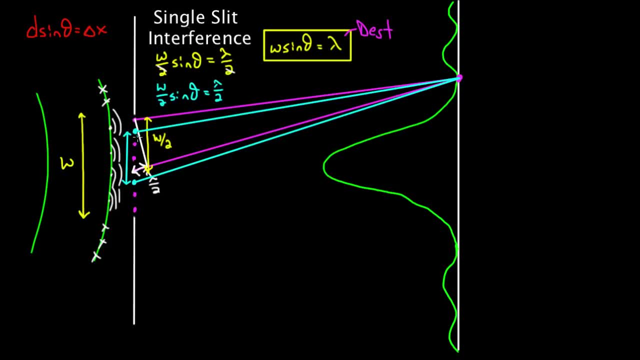 that's also gonna equal half a wavelength. That's also gonna be destructive. These two will also interfere destructively and I can keep playing this game. I can pick this point here over to here and the next one down. These two would have to be destructive. 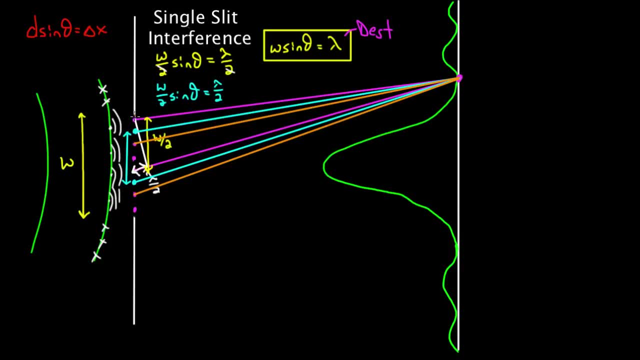 I can pair them off and keep pairing them off. I'd get destructive for all of them. I could annihilate all of them by pairing them off and finding a partner that's destructive to that one, And so this really is a destructive point. 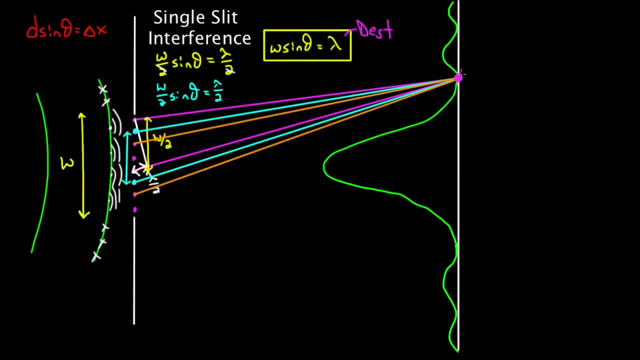 This point over here, all the light is gone, completely annihilated. It gives you destructive. So the short of it is that this relationship here, this relationship that W, this slit, width times sine of theta, the angle, same angle. we've always been defining it as. 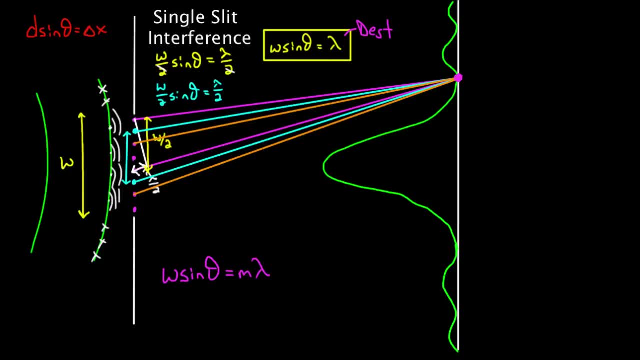 equals integer wavelengths. This time, gotta be careful, though. this time this gives you destructive points, not the constructive points. It was always constructive before. This gives you destructive points now, and you might be upset. You might say: hold on a minute. 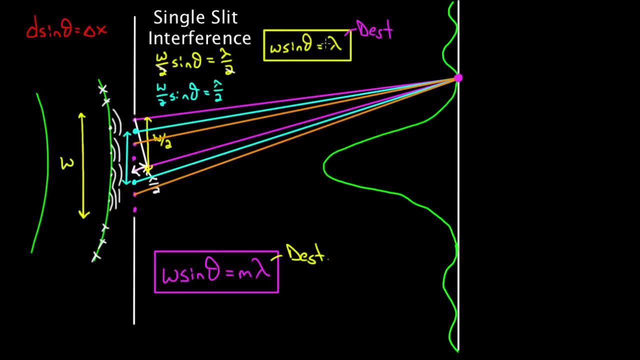 we only proved this, for this was just for n equals one or m equals one, One wavelength. We didn't prove this for anything besides m equals one. Well, you can just as easily show that three lambda over two would also give destructive. 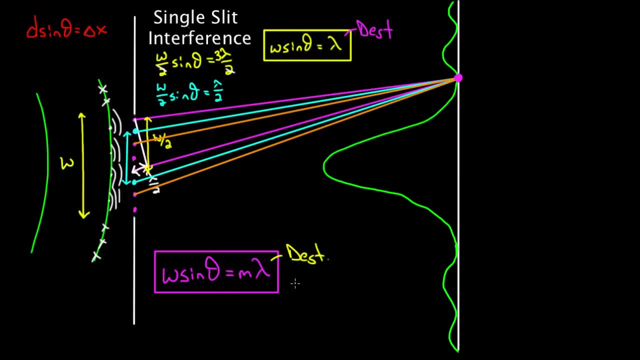 or five lambda over two. that would give us all the odd integers here. So m m here can be. it can't be zero. We'll talk about that in a minute. It could be one, two, three, four, five and so on. 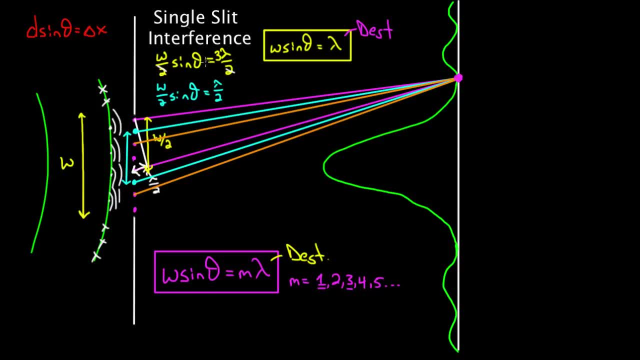 One. we already showed Three. you get well if you made this three halves wavelength. that's also destructive. that'd be three, Five halves wavelength. the twos are always canceling, So five halves wavelength would work. What about the even integers? 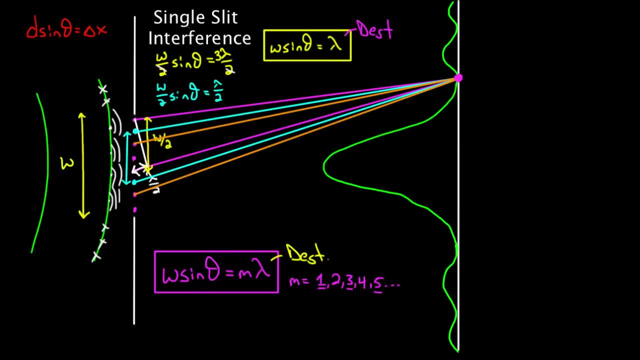 How do we get these? Well, those come from the fact that I didn't have to pair these off with the top one and the middle one. That's dividing this into W over two, So pairing them off by lengths of W over two. 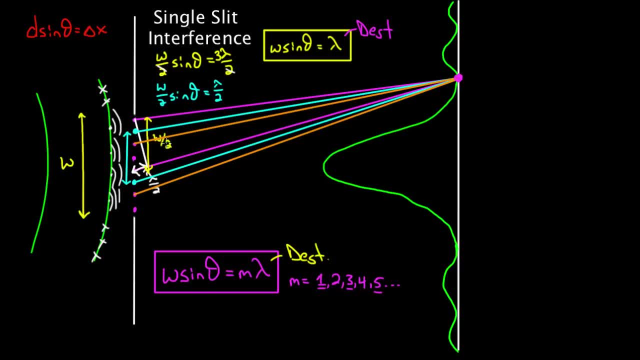 I can pair them off. I can divide this by any, even integer. I can imagine pairing off instead of doing the topmost one and the middle one. I could do the topmost one and skip one down here, And so I can pair these off. 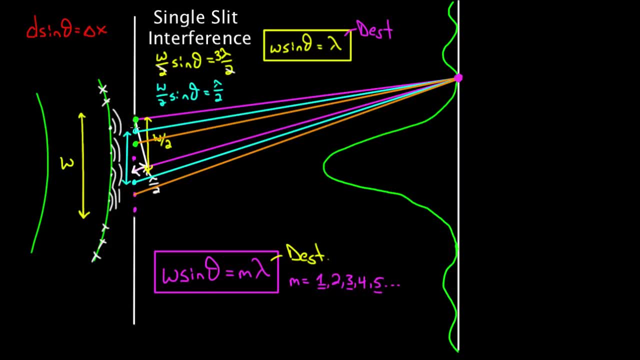 If I divide this into this distance right here, that distance would be what That'd be W over four, And so I can imagine pairing off. okay, if these two cancel, if those two points cancel, then the next one down, so this one here. 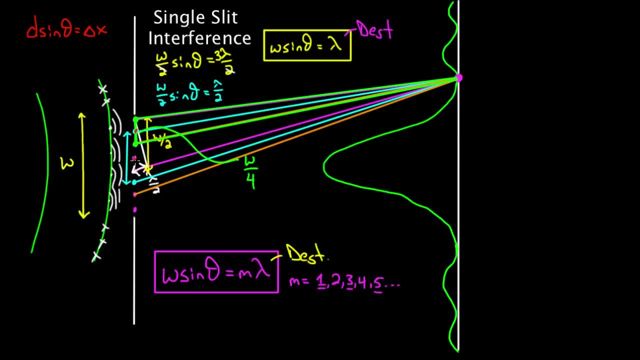 and this one here would also cancel by the same reasoning, And so I can play the same game now, but W over four would be how I divide it. I can't divide it by anything. I can't divide it by three or like 2.5,. 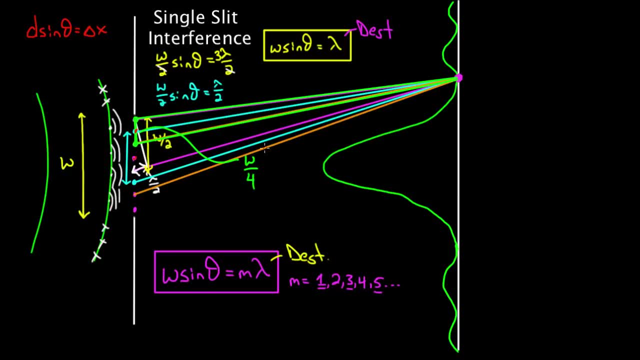 because I always want to pair these off in twos, Always twos. that's my whole plan, That's my whole strategy. My whole strategy here is to cancel these in twos, and I can do that by dividing this by any even integer. 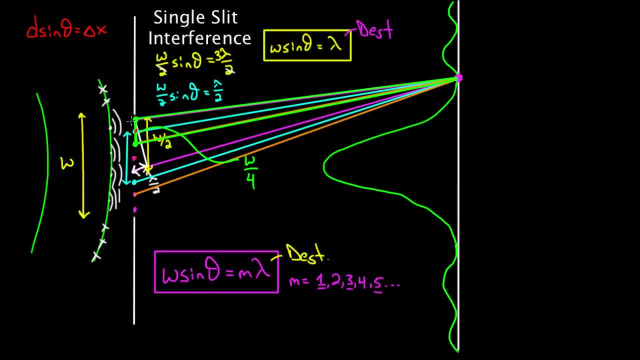 So W over four would work. What would that give us? Okay, W over four is the distance between these times sine theta equals. let's just say it's the first one half of a wavelength. Well, if I solve this, if I move the four over, 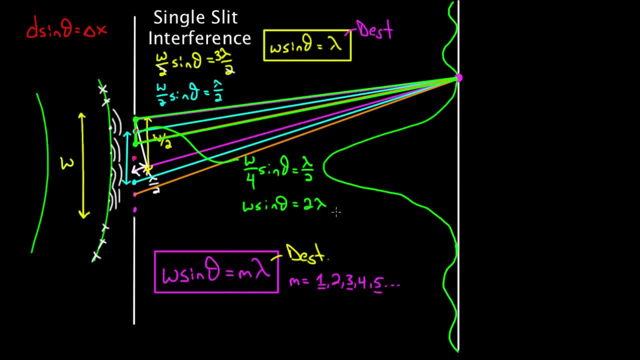 I get W sine theta equals two lambda, So the twos also give us destructive interference. I could divide by eight, That would give us four. Once I move it over, I can divide by any, even integer. Any integer here is going to give us. 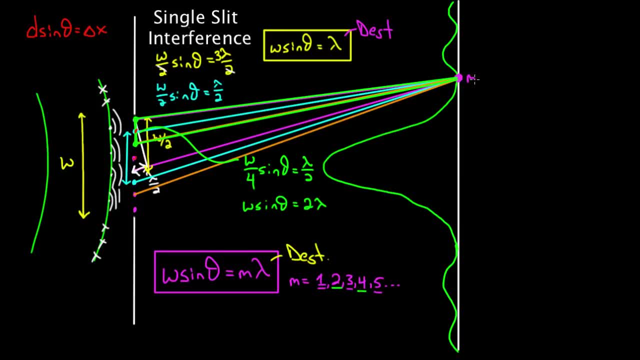 destructive points on the wall. So this would be M equals one, this would be M equals two, and so on upwards. So this relationship right here gives you all the destructive points. How come M equals zero is not a destructive point?